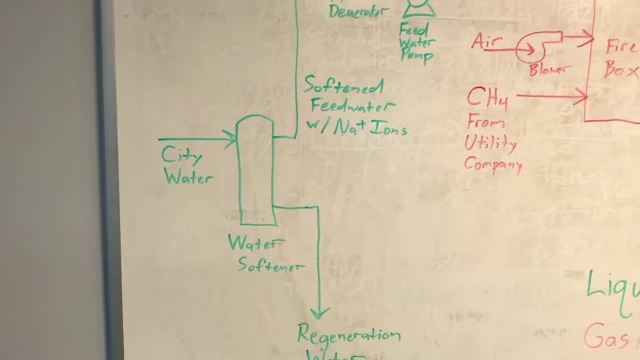 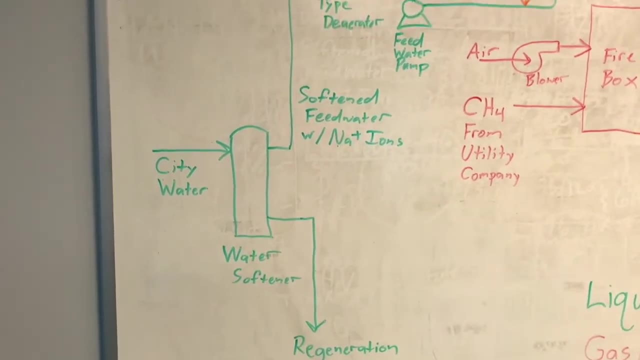 get city water from the city of Lock Haven, It goes through a water softener system. We're not going to talk about a lot of these components in detail. You could research them at your leisure. but the purpose of a water softener is to substitute any of the heavier ions that come in. 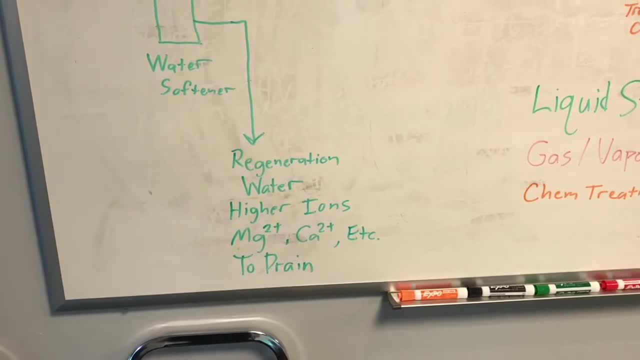 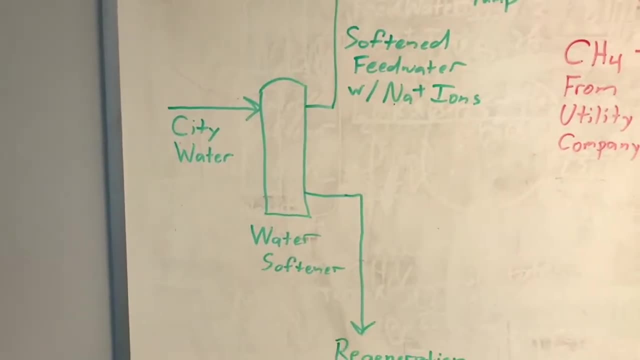 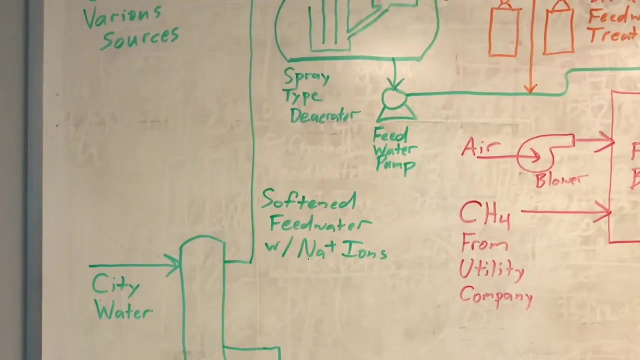 with the city water, such as magnesium and calcium, which cause scaling issues in boilers, and replace them with softened sodium ions. This actually goes through a regeneration purge cycle with a salt brine solution, Which displaces these ions and then moves the softened water through. 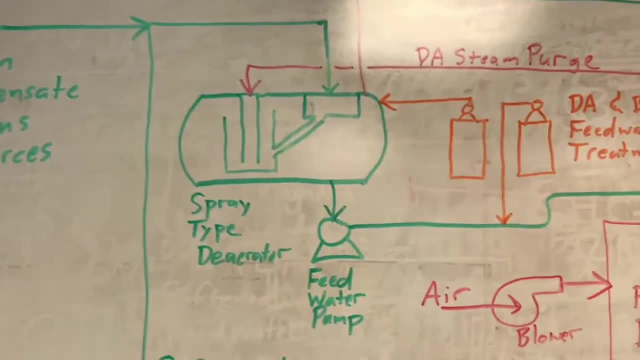 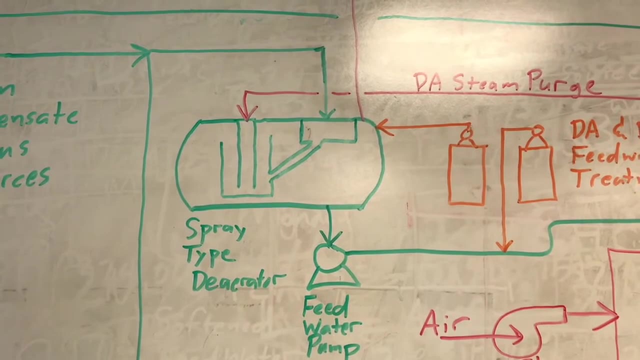 So from there the softened water goes into what's called a deaerator and we have what's called a spray type deaerator where, effectively, the water comes into this tray type thing which drops down into what looks like a bucket and is sparged with steam. 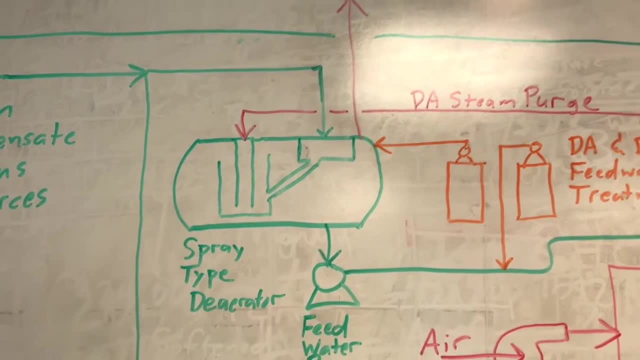 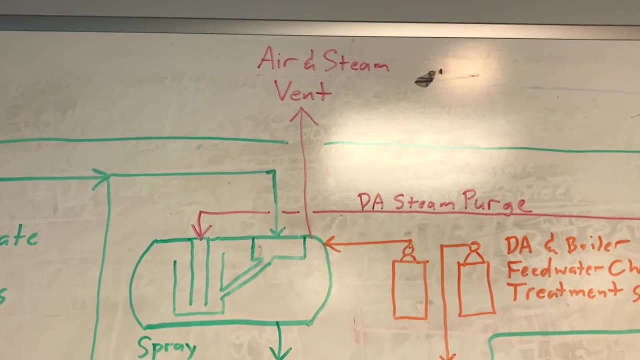 The purpose of that is to heat up the water coming in, to drive off any dissolved oxygen and carbon dioxide which causes the deaerator to degrade. So the deaerator is a spray type deaerator and it's going to cause corrosion issues in boilers through the vent And we'll get back around to the steam. 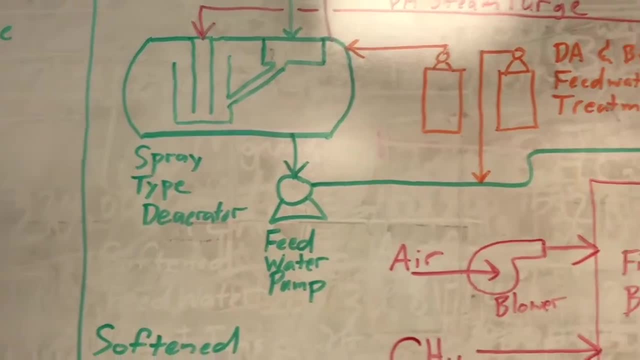 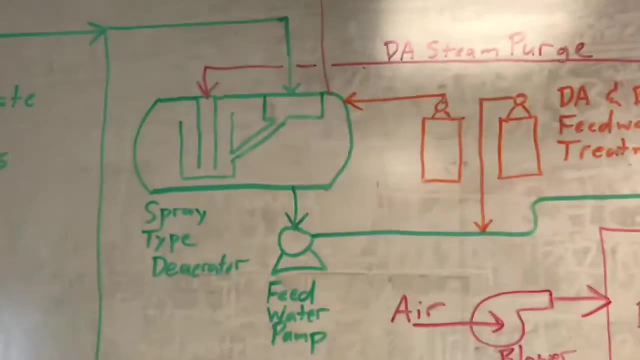 purge later. From there the feed water goes into a feed water pump, which gets pumped into the boiler for boiling and steam generation. In addition to that we have two other smaller liquid streams. Boilers require chemical treatment to prevent corrosion scaling. 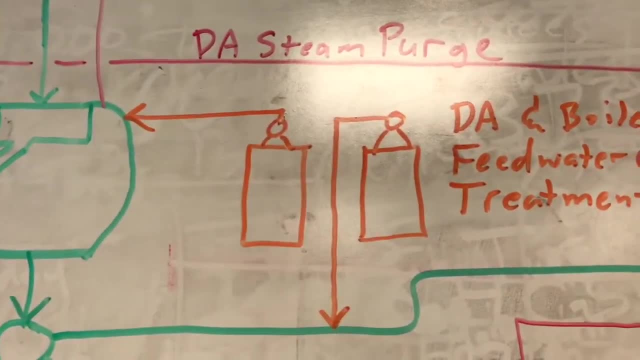 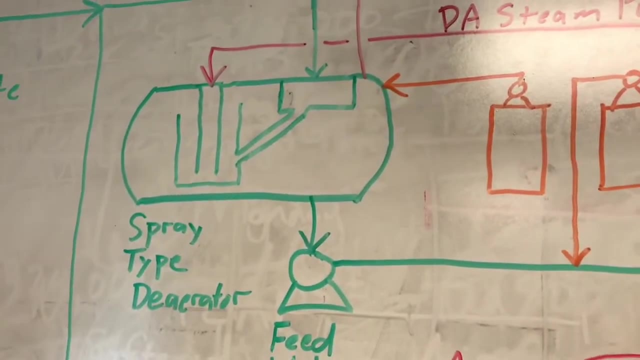 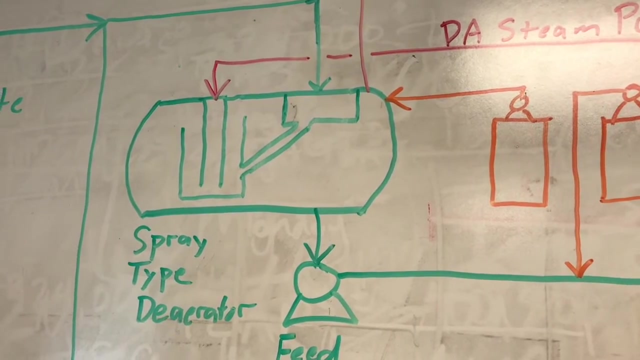 and other problems. We have two. We have a small sulfite solution drum that we have with a small deaerator. That sulfite solution gets injected into the deaerator and the sulfite scavenges any remaining oxygen that the deaeration process doesn't eliminate. And we have another drum. 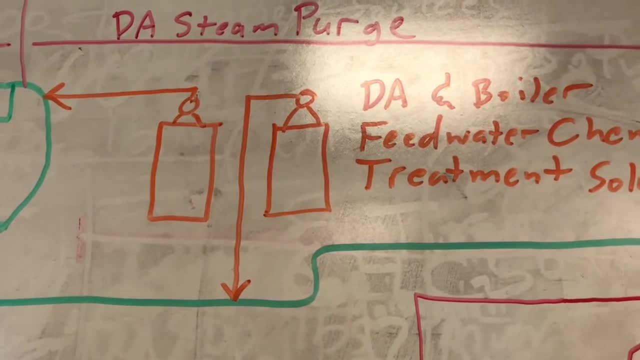 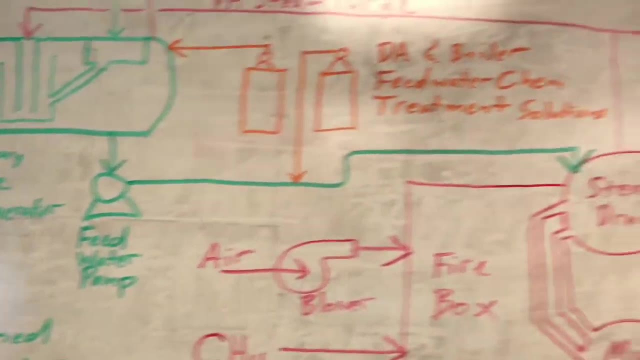 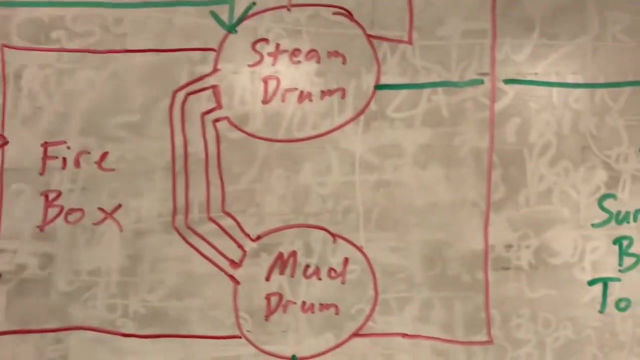 with a cocktail of various ingredients that prevent corrosion scaling other boiler issues, also pH adjustment, as there's a little bit of caustic in it. They get fed into the feed water, which also goes into the boiler and keeps the boiler healthy. Now, from there, water gets boiled. 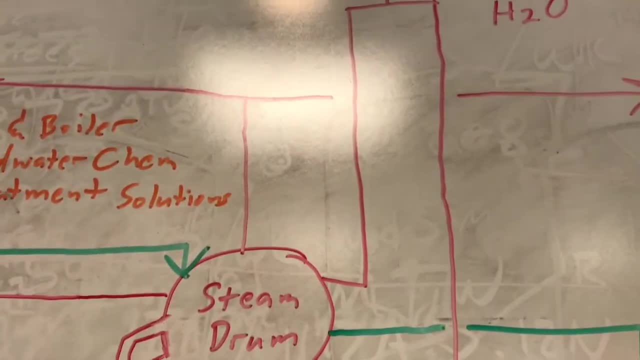 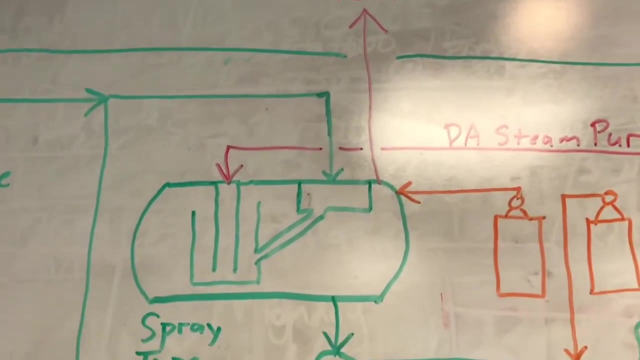 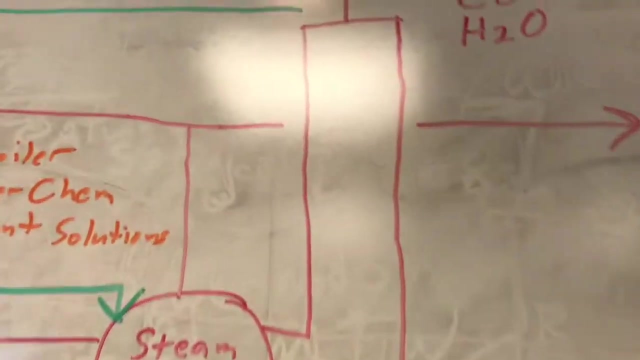 and we have steam generation And in our plant steam goes two main places. We have one stream which purges the deaerator and causes contact through this little scrubber pot system to drive off the dissolved oxygen and carbon dioxide, And we also have steam that goes to all the other. 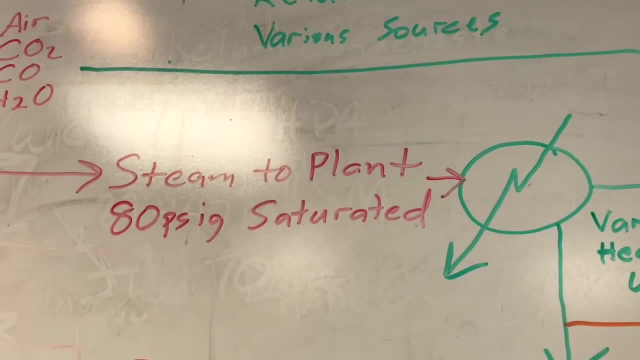 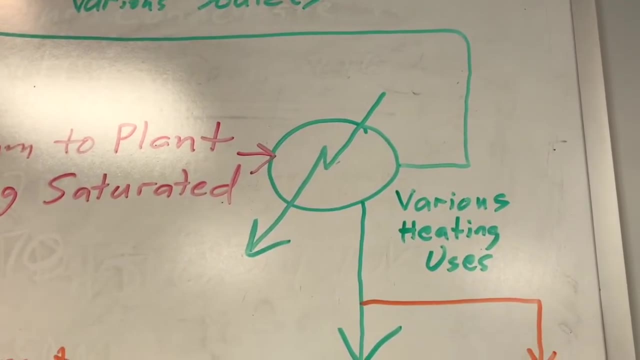 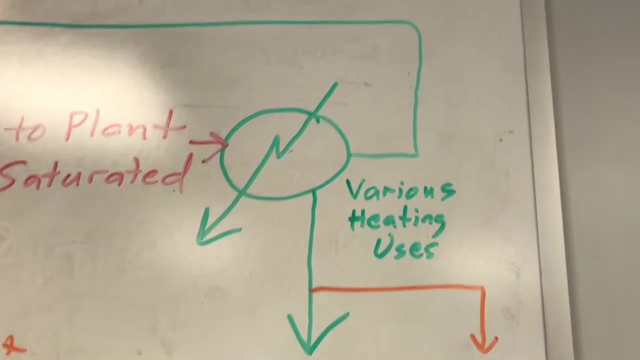 major areas in the plant And the steam we produce in our boiler is 80 PSIG saturated steam. After going through various heating uses it gets condensed into liquid water again and pumped, transferred back to the boiler system or dumped to drain. So we have some streams that are returned condensate. 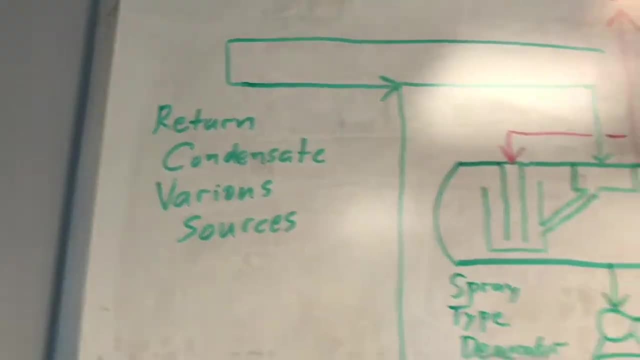 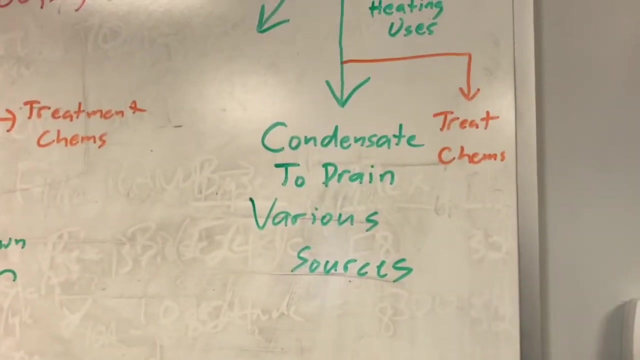 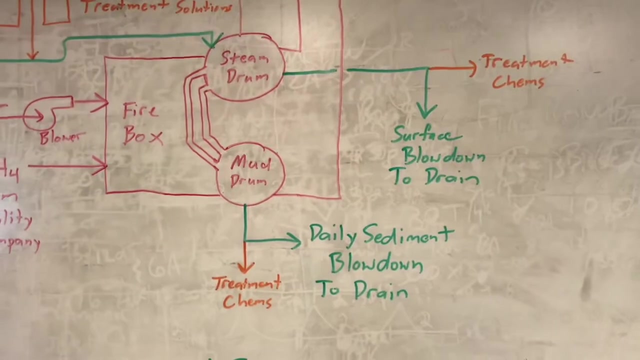 that go all the way back through the plant into the boiler system, along with the feed water, into the deaerator, And then we have some streams which are simply dumped right to the drain. In addition to condensate, there's two other streams that get dumped to the drain. We have what's called blowdown. 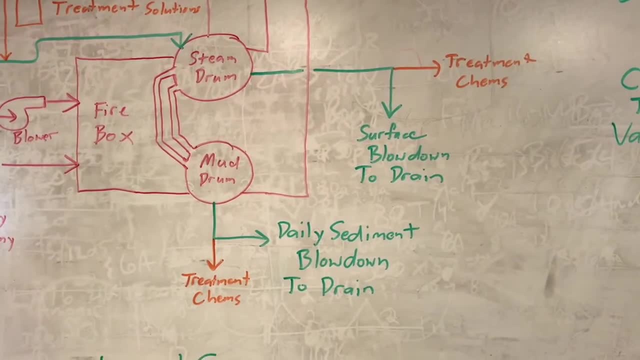 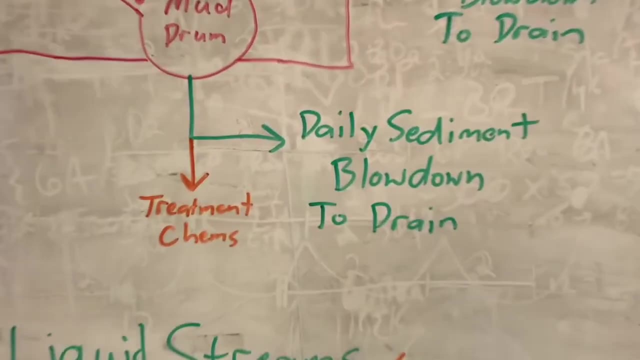 and the purpose of that is to balance the treatment chemicals to make sure they don't build up in the boiler and you keep the proper balance for the concentrations that are needed. We have a daily 30 to 60 second sediment blowdown where we purge the water out and any dirt that may. 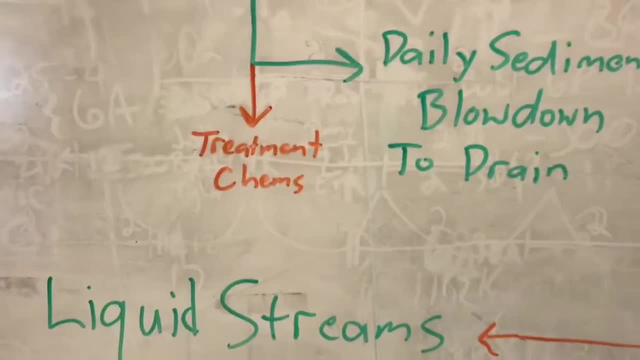 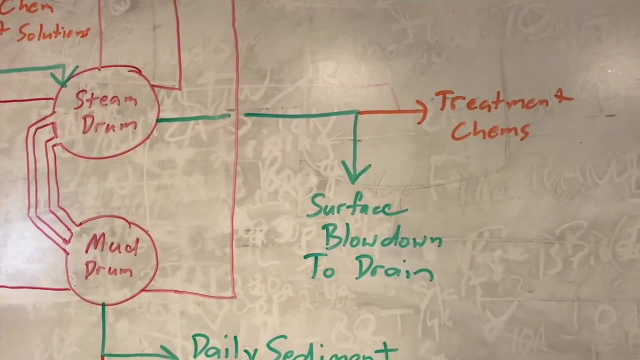 be collecting in the mud drum, as we call it. We also have a small amount of treatment chemicals that come out with it. We also have a surface blowdown, which is a very small half inch line continuous flow, which is a very small half inch line continuous flow. 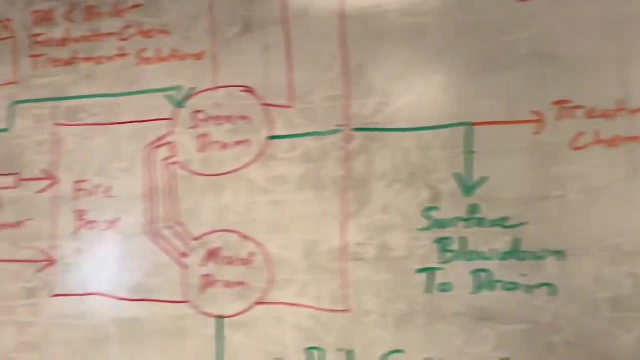 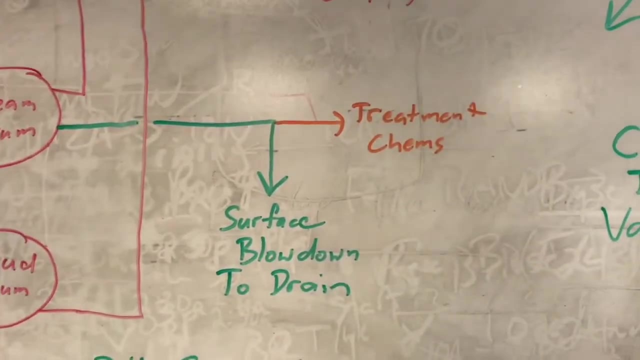 The main purpose of this is to balance the treatment chemical concentration in the boiler to make sure we don't have an excess and we don't have too much. So this takes a little bit of trial and error to get that. but if you sample and analyze for your treatment chemicals you can figure out quite easily how to balance it. 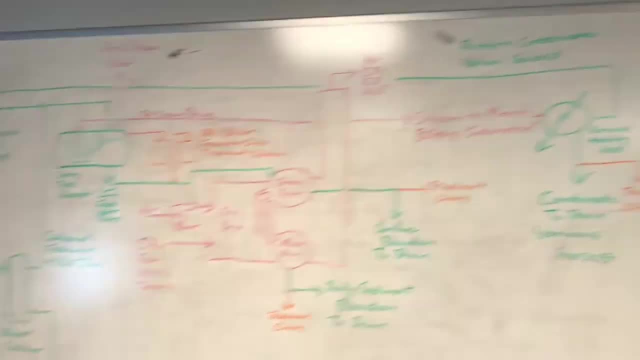 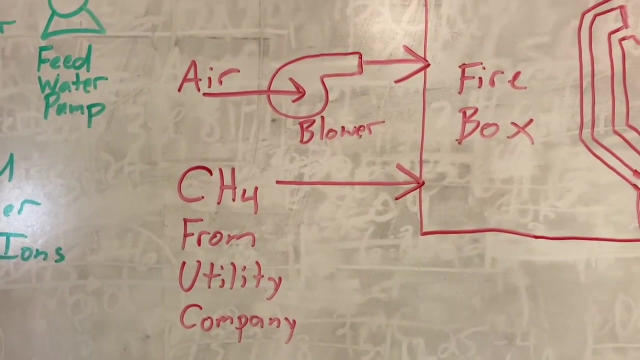 So that pretty much goes over all the liquid streams. Now let's talk about the combustion side. Very simple: We get natural gas from our utility company, which happens to be UGI. We also get combustion air, which comes right in from the atmosphere with a blower. 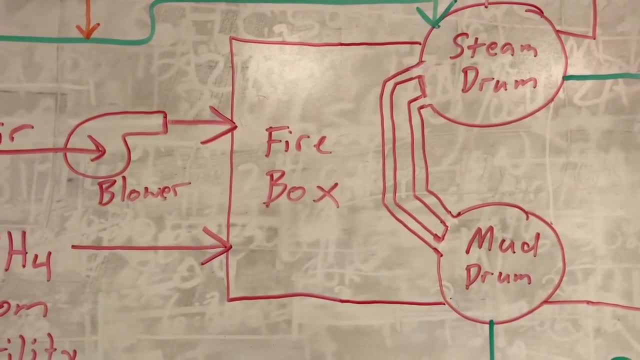 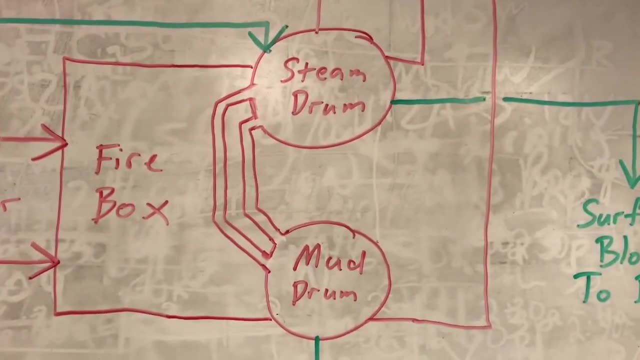 Those two get mixed in the firebox and obviously there's a burner in there, creating the flame and the heat. That heat passes over the tubes of our water tube boiler and then the liquid that's contained in the mud drum and part of the steam drum gets boiled. 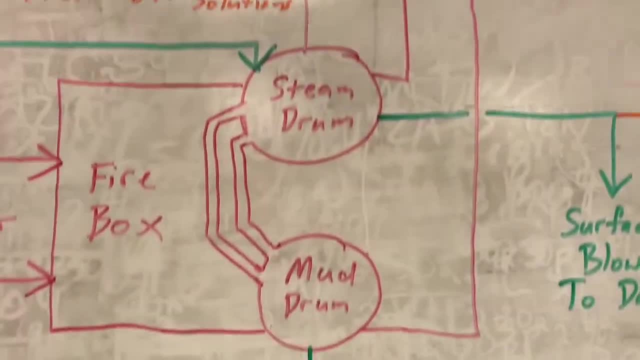 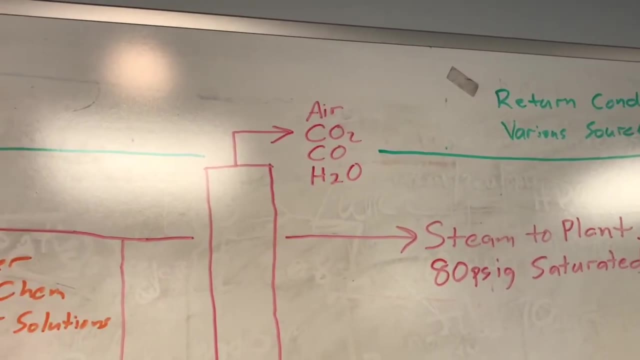 given off the steam, as we already discussed. Then the combustion gases come out the boiler stack in the roof of the boiler room, where we have some excess air, carbon dioxide, meat and maybe some carbon monoxide and water vapor from the combustion reaction. 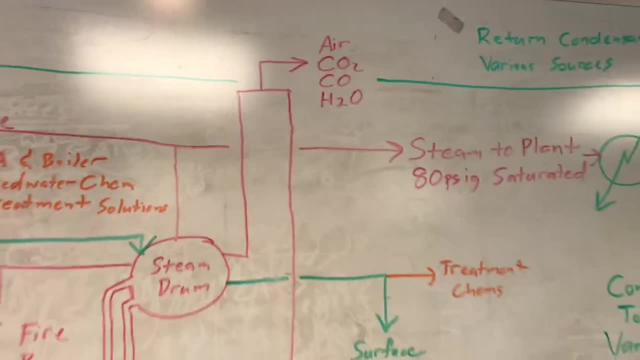 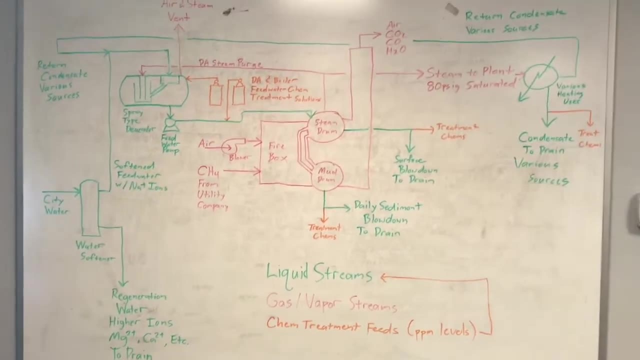 We could spend days and weeks talking about boiler efficiency, combustion efficiency, so on and so forth, but we're just here to give you a general idea of what's going on. So now that we've gone over that, let's go take a walk out in the field and see the boiler system in real life. 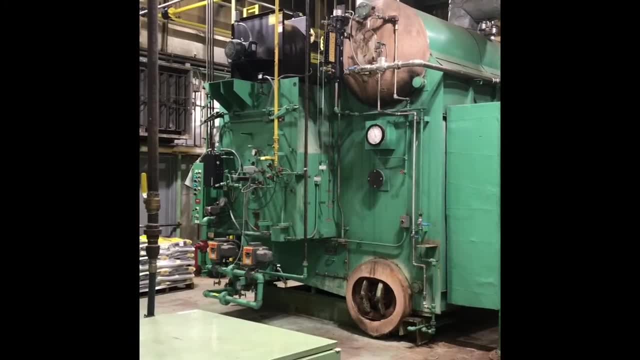 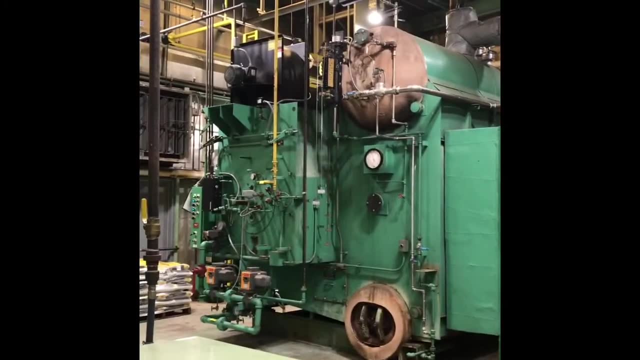 So here we are in the boiler room. You can kind of put a visual diagram that we just reviewed Right. here is the plant boiler. This is a water tube style boiler And we're going to go ahead and kind of walk through the different components of the system. 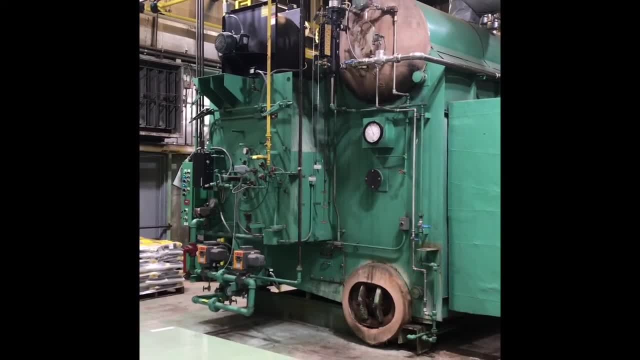 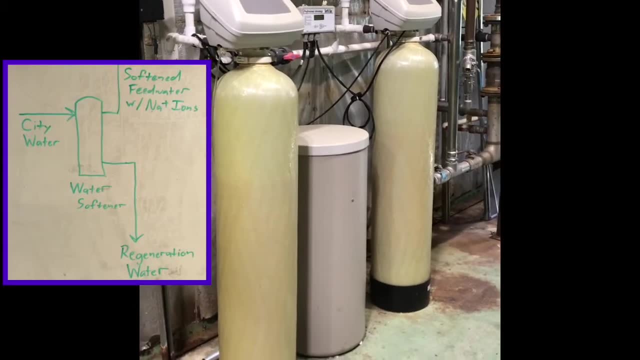 that will follow right along with the process flow diagram. Here's your very first input stream, which is the actual feed water that goes to the boiler deaerator. This is a small water softener system, actually kind of similar to what you might find in a home. 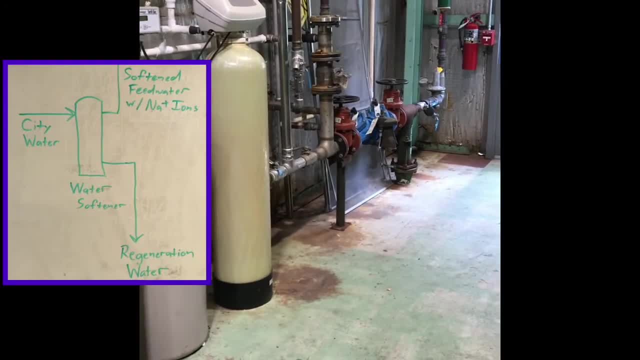 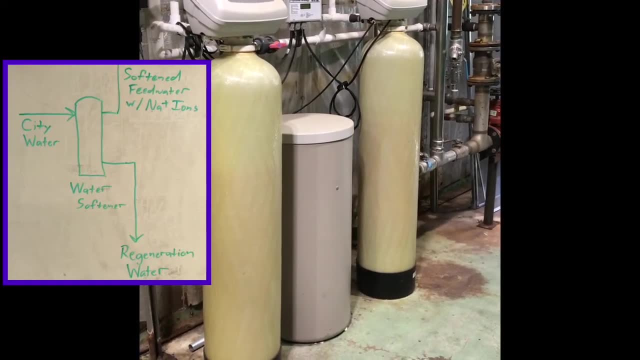 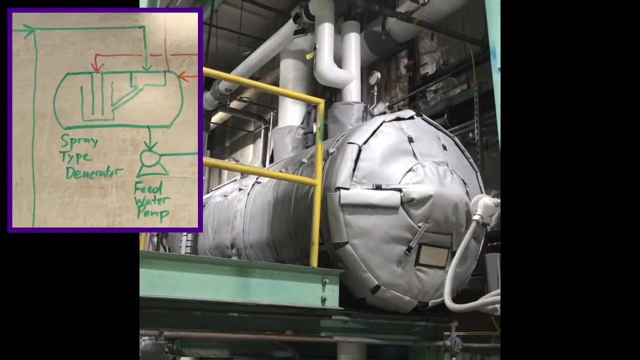 Basically city water from the city of Lock Haven comes in And it goes through the softener system And the higher metals exchange with the sodium ions to soften the water And from there it goes to the actual deaerator. So here is the deaerator for the boiler. 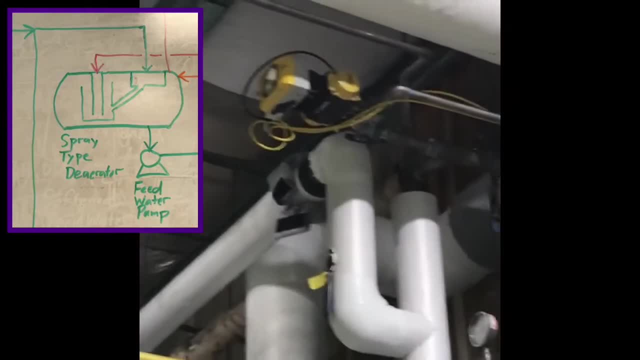 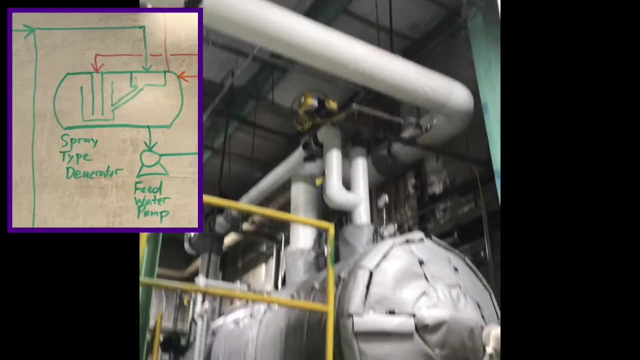 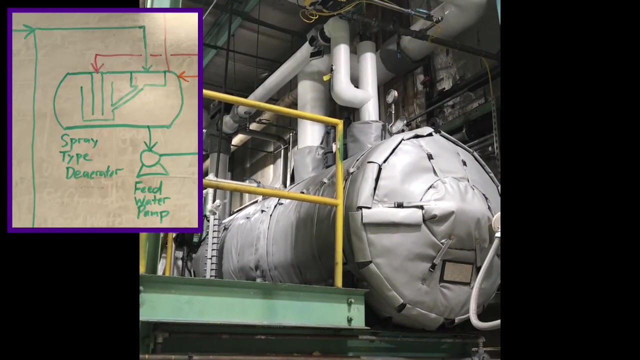 And if you look up here, if you zoom in, that is the control valve that regulates the flow of the feed water. in Feed water goes into the top of the deaerator and down through a little scrubber column. Steam contacts the feed water and helps to evacuate all the oxygen. 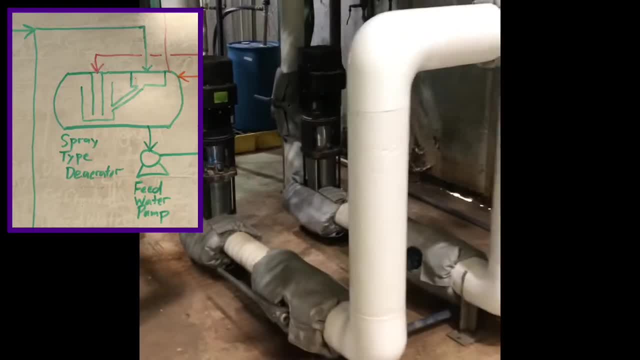 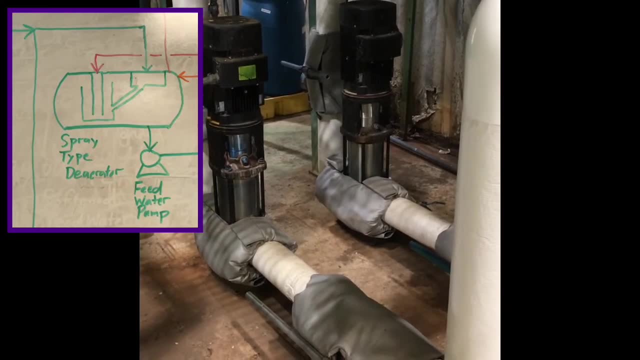 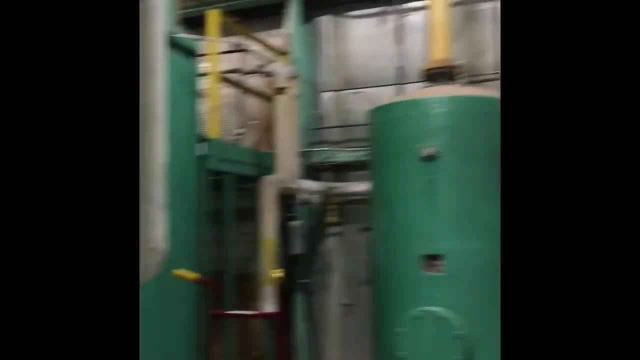 And from there the feed water goes to the feed water pump. The feed water pump triggers on and off as the boiler calls for water. From there, the transfer line progresses up through the boiler room, down through a series of check valves to prevent backflow. 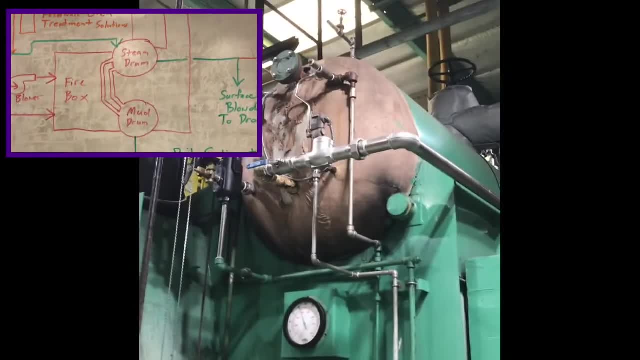 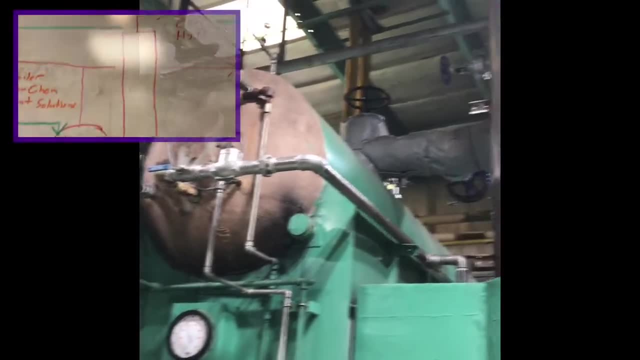 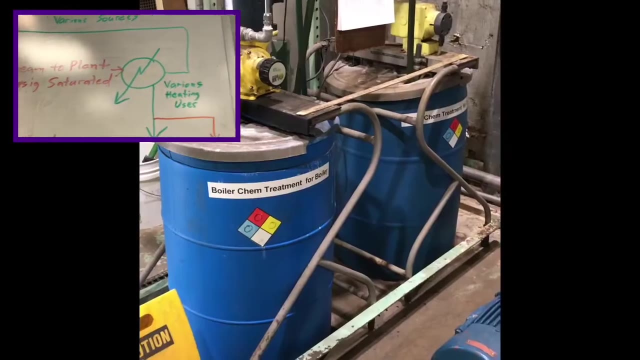 And then finally up into the deaerator And up into the boiler steam drum. From there water gets heated, It enters into steam, It exits through the main steam header To various different areas of the plant. Here is two of our smaller input streams for the boiler system, which are the treatment chemicals. 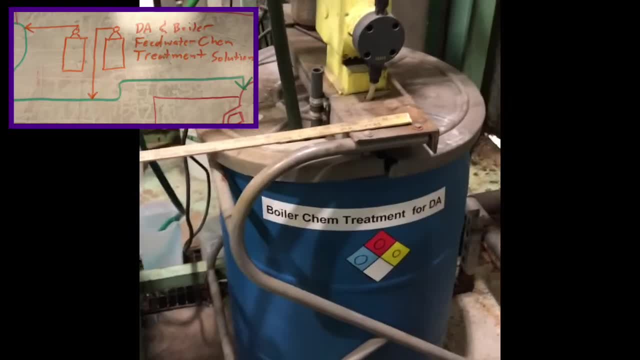 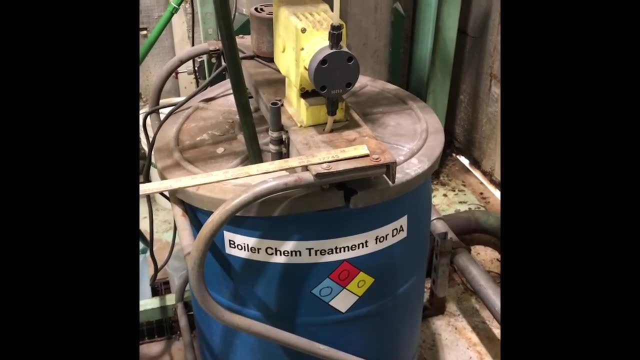 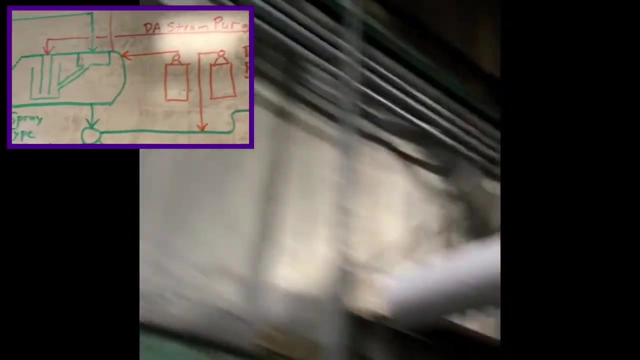 We have two. The first one here is a sulfite powder, And the purpose of the sulfite powder is to help tie up and chemically consume any of the oxygen that doesn't get driven off by the deaerator system, So that slowly gets fed and dosed directly into the deaerator and gets carried over with the boiler feed water. 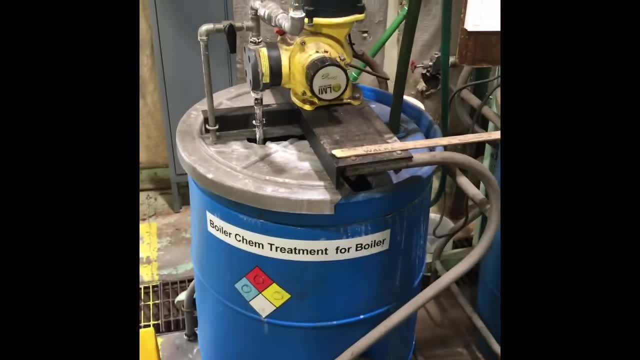 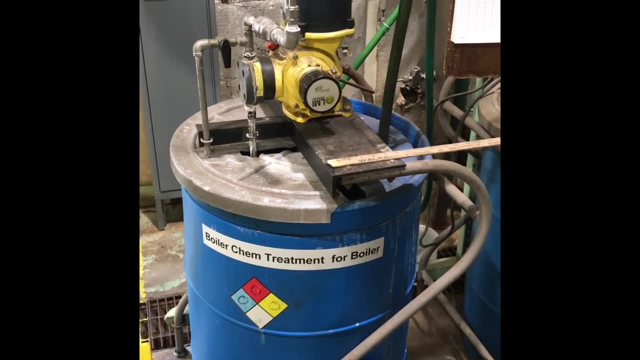 The next treatment chemical we have is kind of an all-in-one cocktail for boiler treatment with an erosion inhibitor, anti-scaling agent and all kinds of other good stuff. We get these from various manufacturers that make water treatment chemicals From here. it gets dosed from the makeup drum. 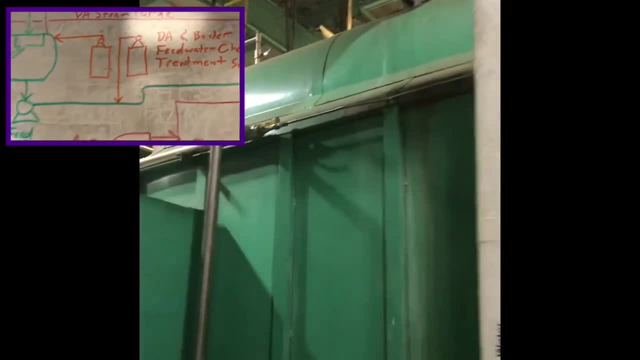 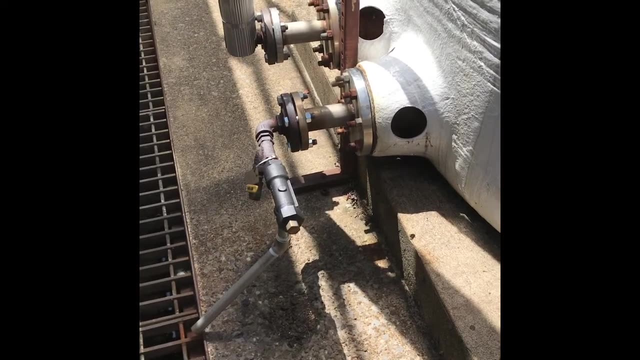 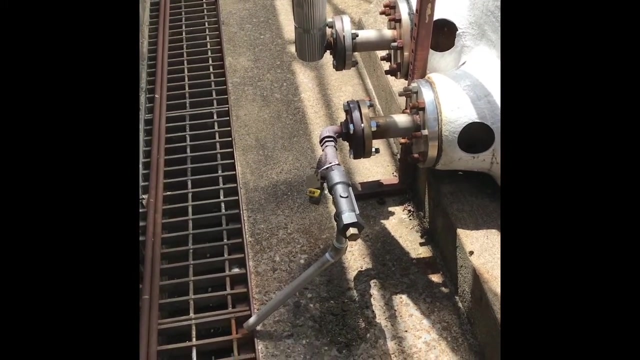 Up and directly into the boiler feed water line On its way into the boiler. So as we continue on our path of the water which goes from feed water to steam, out to plant distribution, we have two situations then. One, for example, like we have on this wastewater tank. 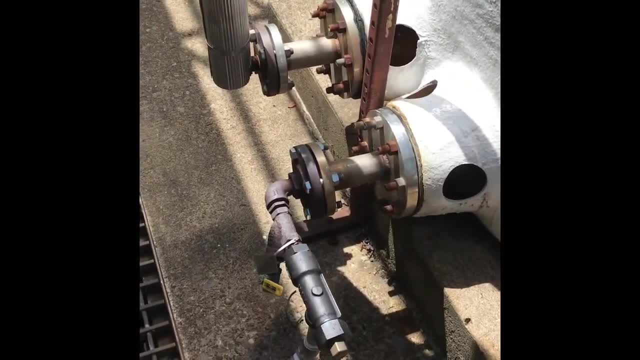 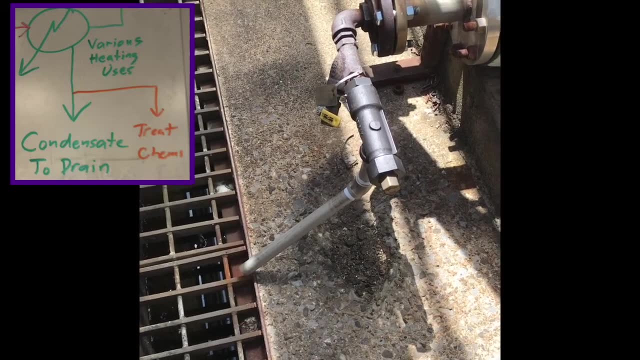 is. steam goes into the heating coil to keep the wastewater warm in the wintertime, But in this particular case we dump it right to the drain and it goes to wastewater. So some of the water that gets converted into steam ends up just going right down the drain. 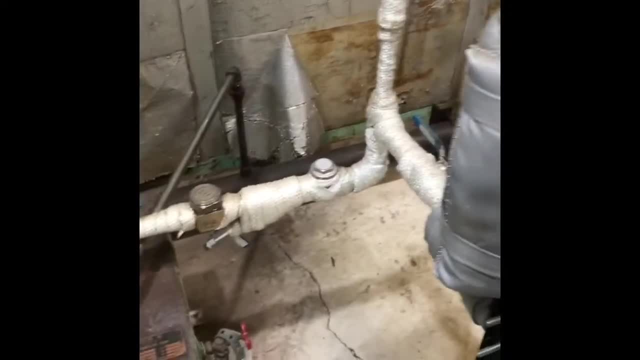 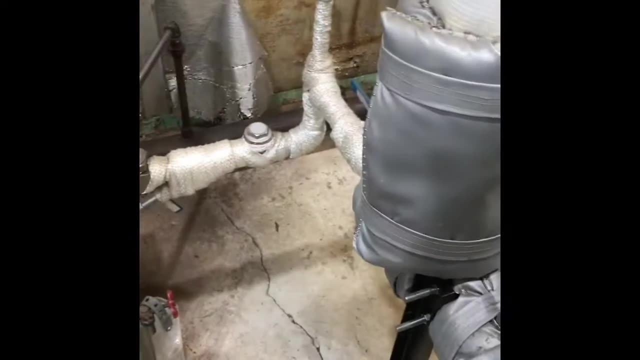 And again in other situations. sometimes the steam gets condensed through various heating processes and then collected, Like in this example here, where the steam condensate gets collected into a small tank And then from here the tank actually gets pumped back into. 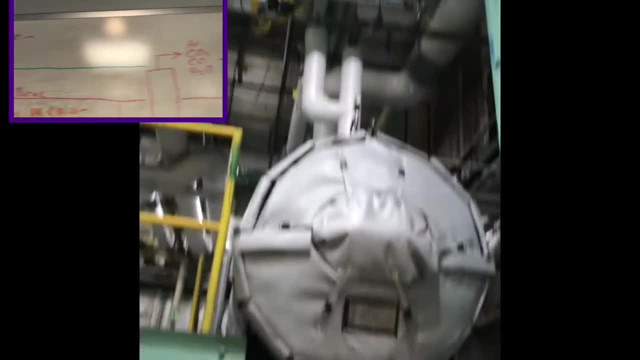 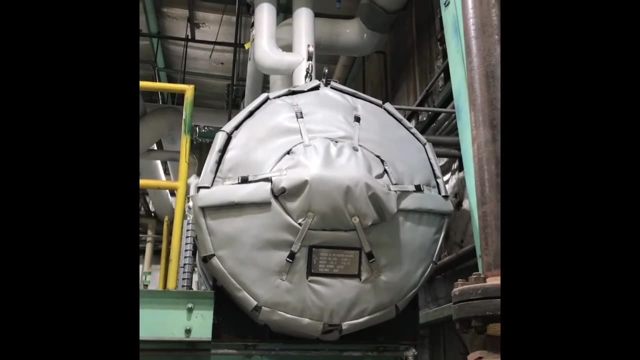 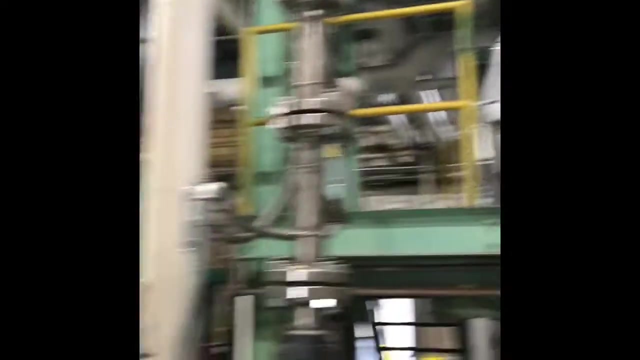 a piping distribution series. It goes right back into the area. So we have some steam that gets wasted after it turns into condensate And we have some steam that gets collected into condensate and returned in a recycle loop right back into the boiler. 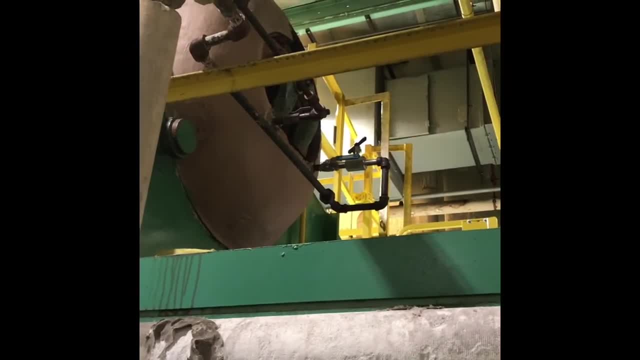 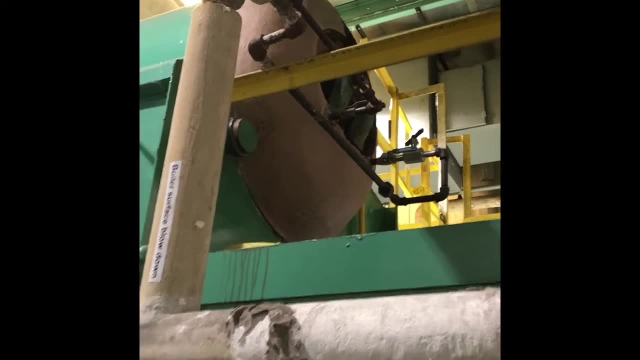 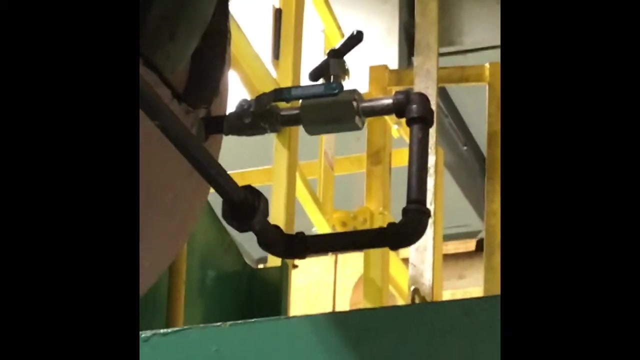 We also have two very small waste streams from the boiler. that's required, So chemicals and also conductivity creating elements doesn't get collected into the boiler. We have what we call a surface blowdown, which has a small valve that's continuously cracked to bleed just a little bit of water out of the boiler and into our blowdown drum. 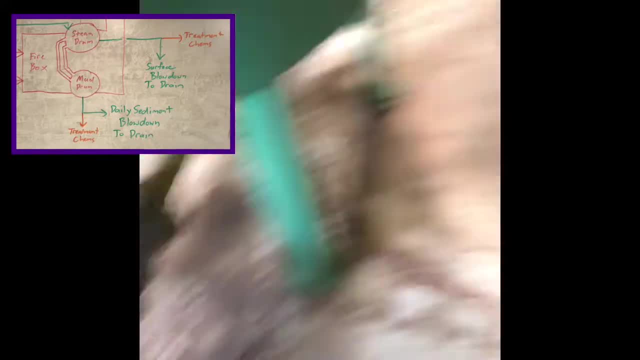 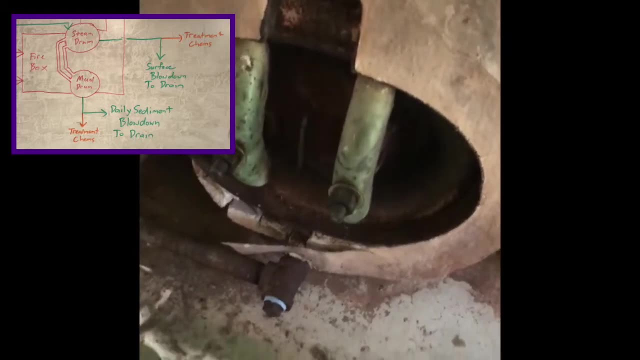 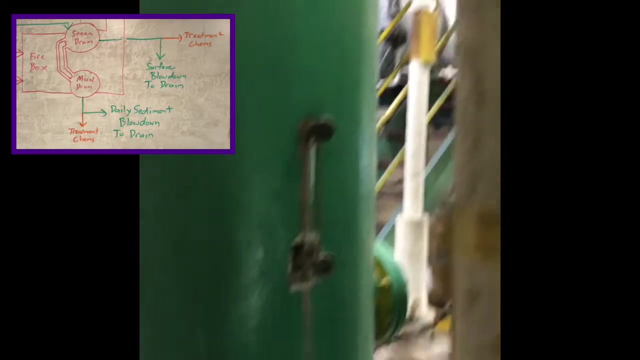 straight down to the drain And then, once a day for about 30 to 60 seconds to remove any sediment that's collected on the bottom mud drum of the boiler. we open our blowdown valves, blow out down for about 30 seconds to a minute to evacuate any sediment in the bottom, which also goes. 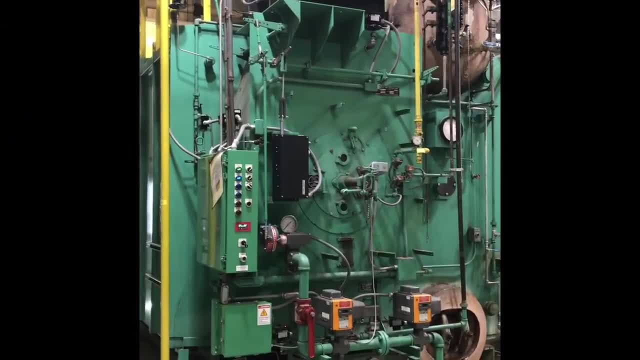 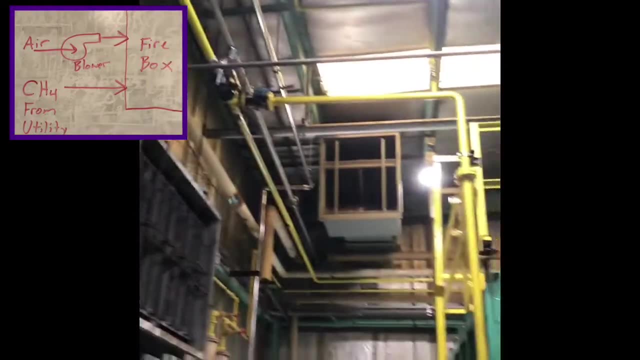 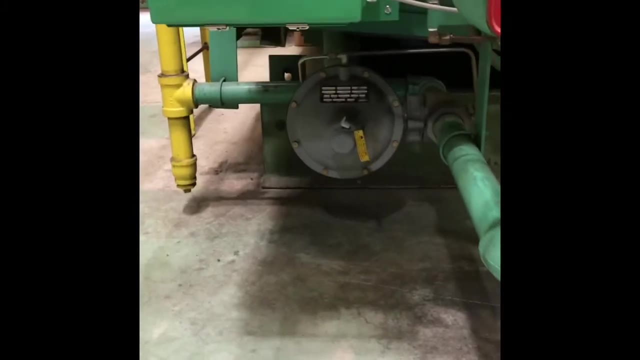 right down the drain. So that concludes the walk-down of the water side of the boiler. Now let's look at the combustion side of the boiler. So we have natural gas from the utility company that comes into the boiler room. It goes through a series of pressure reducing regulators to drop the pressure. 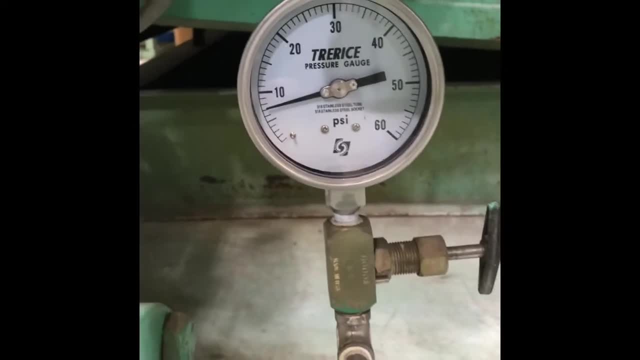 So the pressure of the natural gas coming into the boiler is going to go through the boiler. The actual pressure of the natural gas coming into the boiler is only about 6 psi. From there it goes through a series of safety valves which shut and kill pool in the boiler. 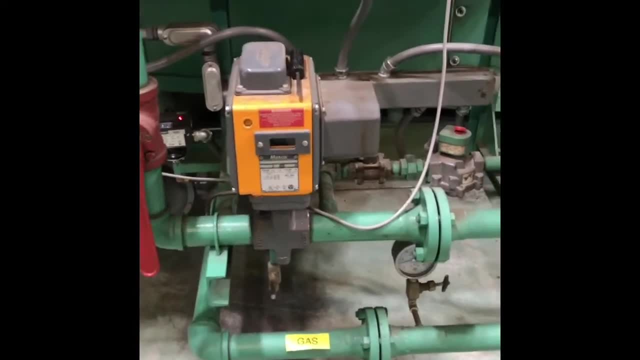 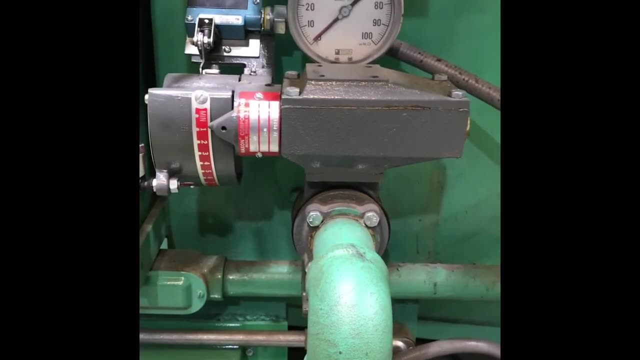 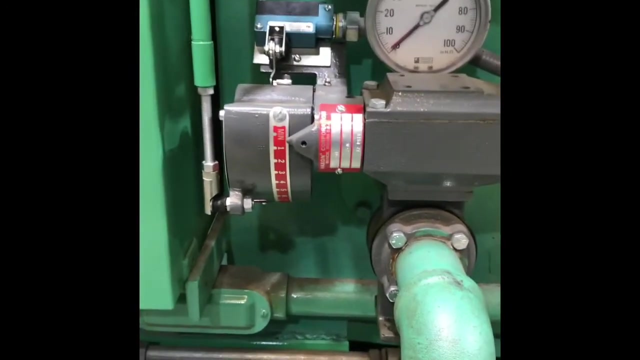 in case any issues occur. From there, the natural gas goes through a control valve which regulates the flow of natural gas into the boiler for heating demand requirements And in this particular case, right here, we have very low demand, as we're on the minimum. 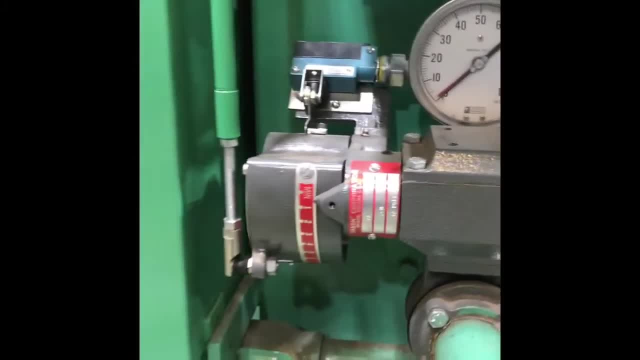 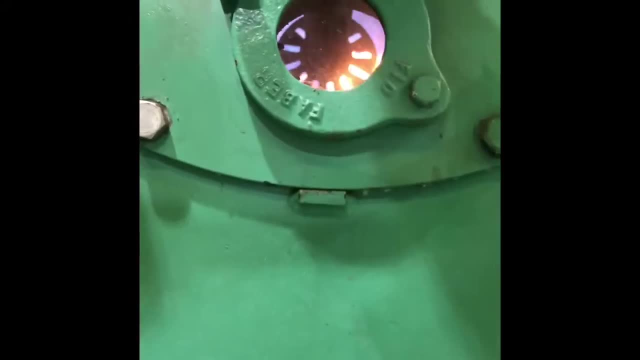 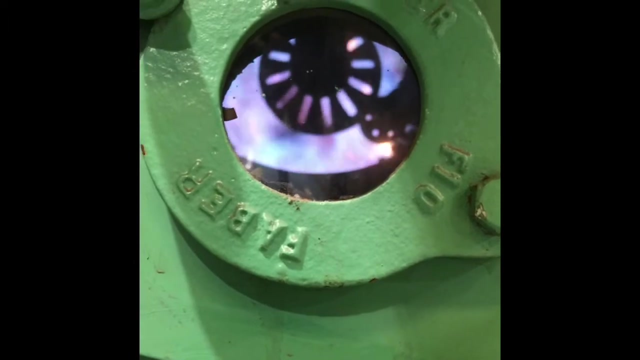 setting and lowest feed pressure, And then you've got a low-speed pressure- It's about 10 horsepower and that's the same as the power- And from there the natural gas goes into the boiler, into the actual combustion chamber, which we have a nice ceiling window of, where it gets heated and reacts with the oxygen. 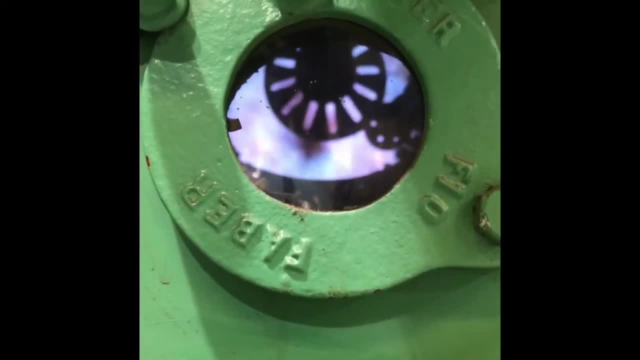 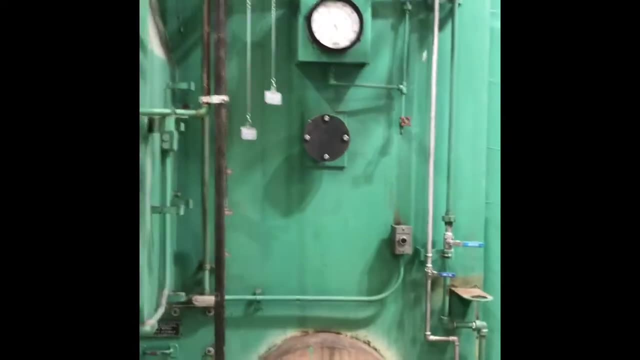 in the air. We have a basic natural gas-oxygen-combustion reaction which provides the heat. This then heats the tubes of the water tube boiler, so the tubes actually extend kind of in this shape right here from top to bottom. 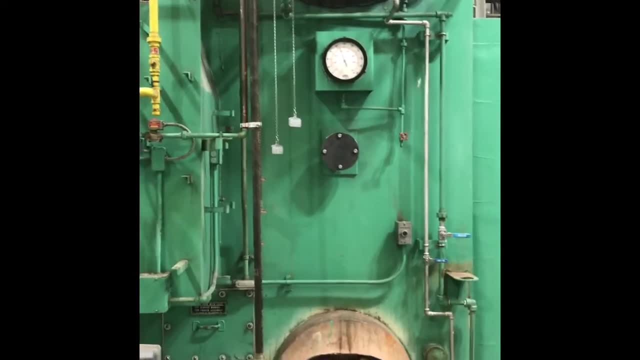 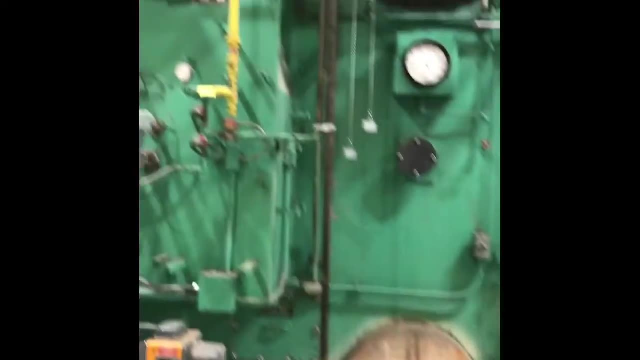 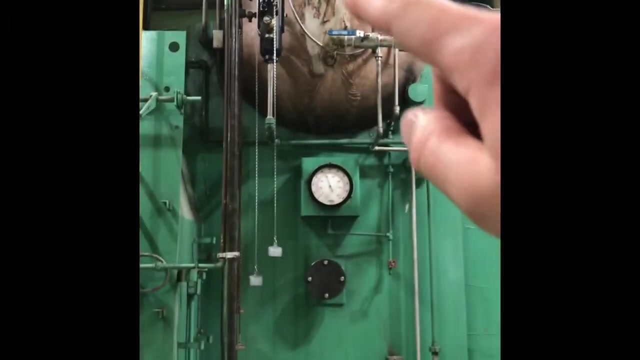 If you look up the water tube boiler you'll see various examples: The lower drum they call the mud drum, which we talked about, where the sediment collects and gets blown out And then, as the tubes get heated by the natural gas, it then boils up into the steam drum. 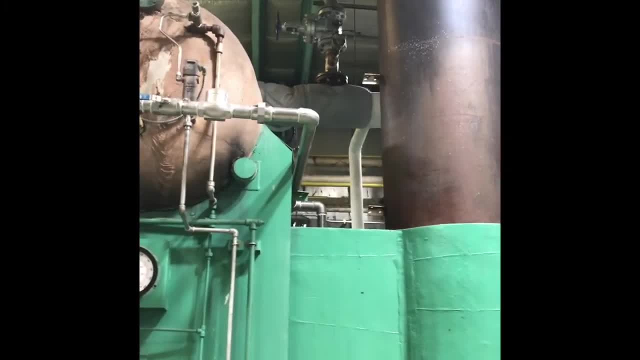 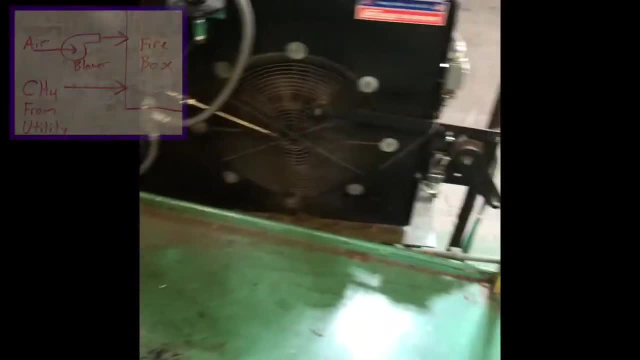 The steam comes off the top into the steam distribution header which we saw in our water sidewalk. So now we're standing on the very top of the boiler where it's boiling. It's quite warm. The air for the combustion reaction comes in through the combustion fan.